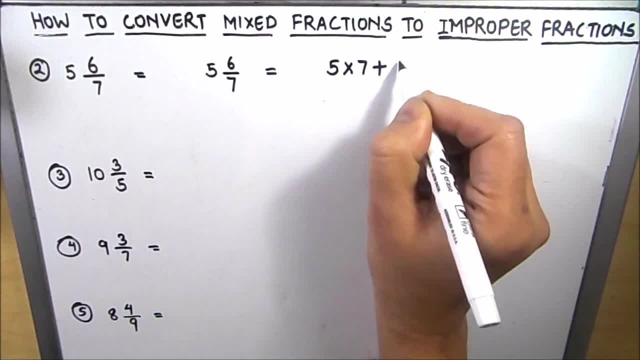 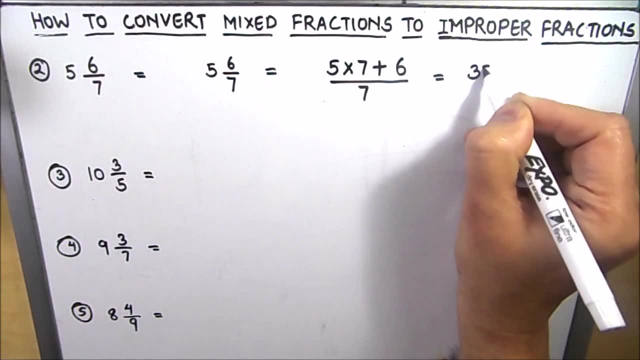 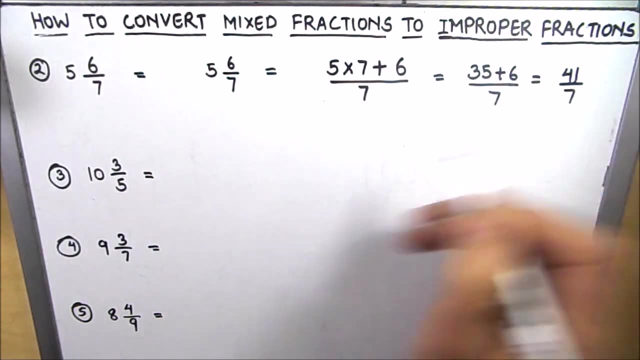 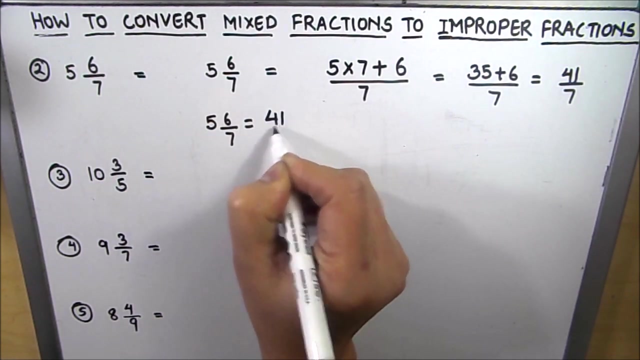 divisor plus remainder, which is the number in the numerator over 7.. So this will become 35 plus 6 over 7, which will give us 41 over 7.. So 5, 6 over 7 in mixed fraction is equal to 41 over 7 as improper fraction. 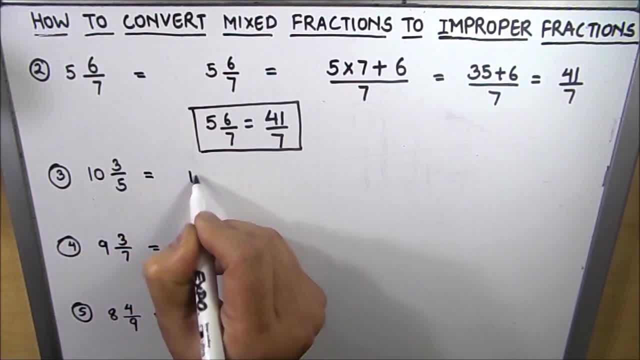 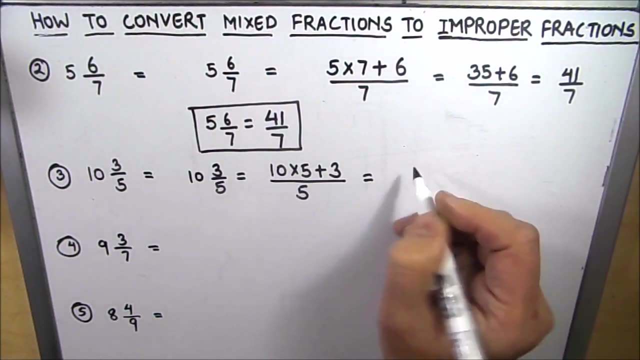 Now. next, we have 10 3- 5's To convert. we have to multiply the quotient and divisor, So 10 times 5 plus 3 over 5.. This is going to give us 50. Plus 3 over 5, which is equal to 53 over 5.. 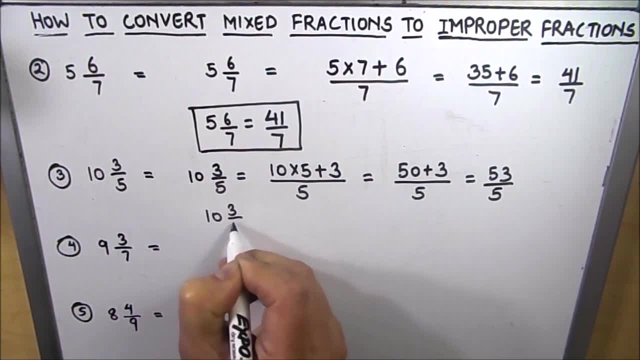 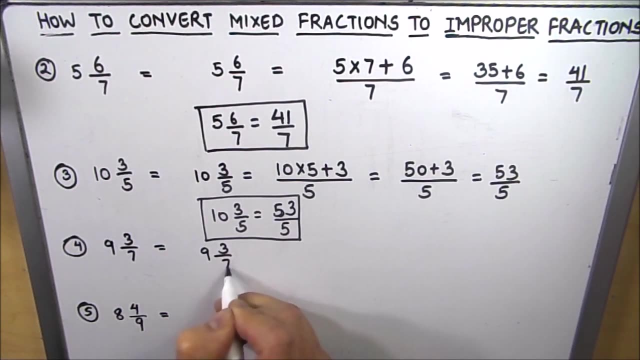 So 10 3 5's is equal to 53 over 5.. Now next is 9 3 7's. This can be written as 9 times 7.. Plus 3 over 7, which is going to give us 63, plus 3 over 7, which is going to give us 66 over 7.. 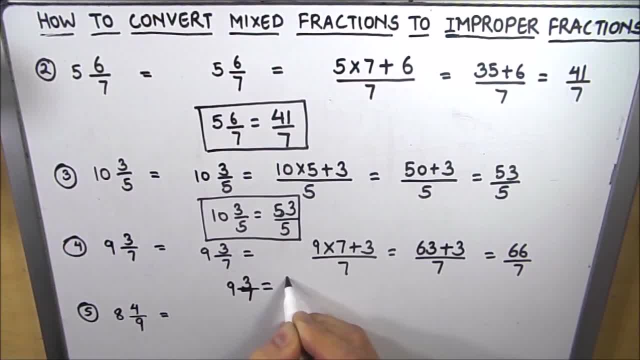 So 9 3- 7's is equal to 66 over 7.. Now here comes the last mixed fraction, which is 8: 4- 9's. So here we are going to multiply 8 by 9 plus 4 over 9.. 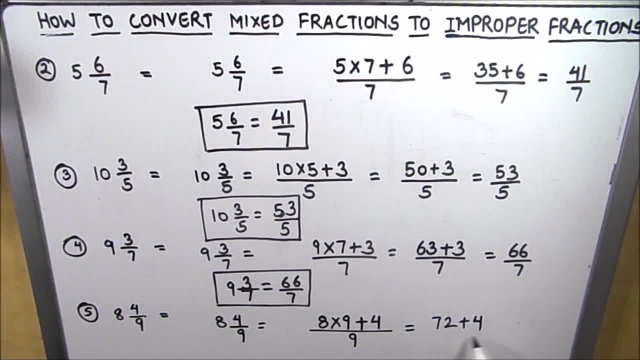 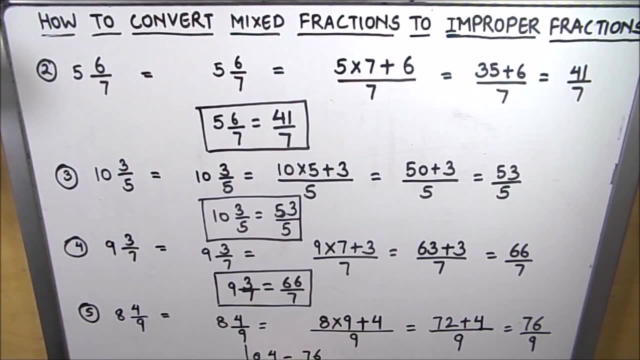 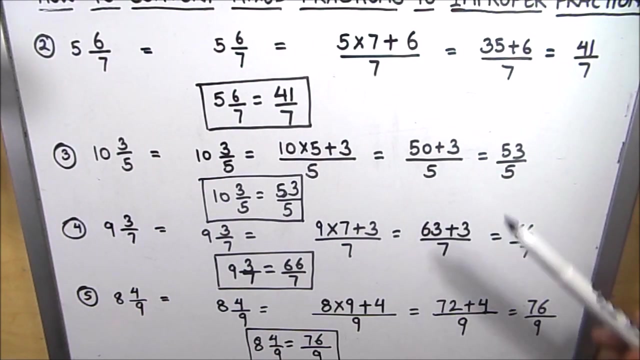 So this is going to be 72 plus 4 over 9, which is going to give us 76 over 9.. So 8 4 9's is equal to 76 over 9.. This is the final conversion. So I hope that by solving these examples with me, you can now easily convert any mixed fraction to improper fractions. Thanks for watching.